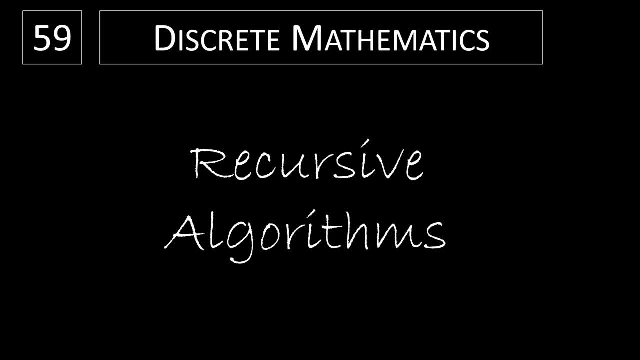 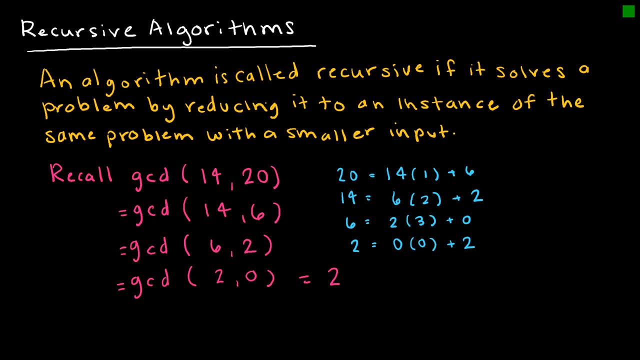 Let's finish off our study of induction and recursive definitions with a little bit of knowledge of recursive algorithms. So we're going back to pseudocode. So a recursive algorithm is basically an algorithm that solves a problem by reducing it to an instance of the same problem with a smaller input. So it just keeps doing that over and over. 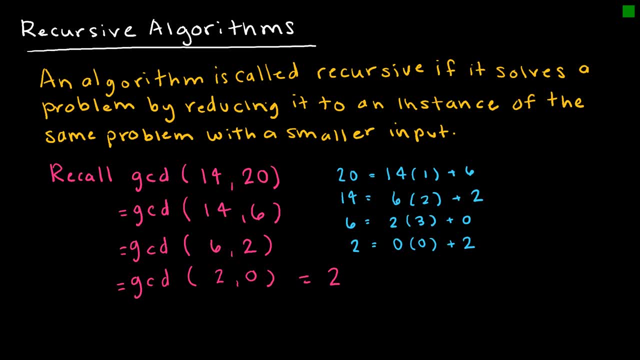 So I wrote down an example that should look familiar to you, using the Euclidean algorithm that says: hey, if I wanted to find the GCD of 14 and 20, then really, what I'm doing is I'm saying: let's take 20 and make it equal to 14 times whatever number, plus the remainder, which of 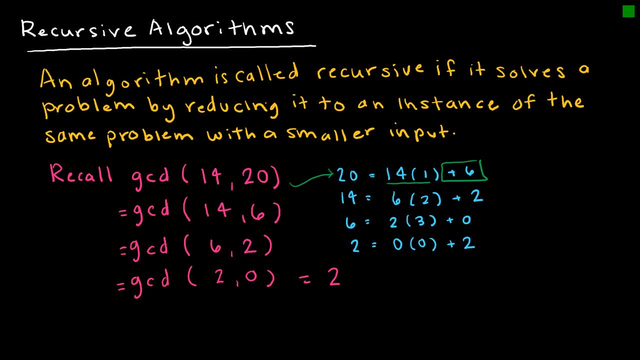 course means that mod right, So mod would be 6. And then I can rewrite that as the GCD of the smaller number and the GCD of the smaller number, And then I can rewrite that as the GCD of the whatever the remainder was. So that's equal to the GCD of 14 and 6.. So now I'm dealing with the 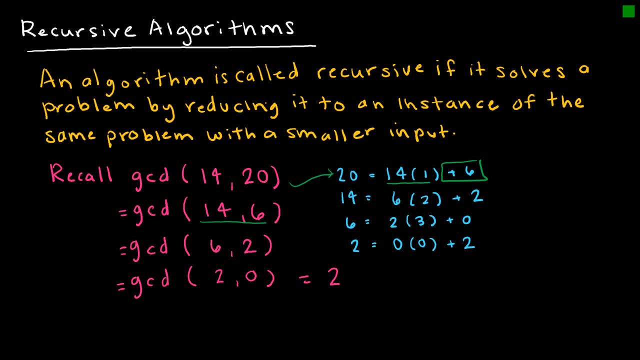 same problem but smaller inputs. And then I repeat that process and I get 6 and 2.. And then I say well, okay, that's equal to the GCD of 6 and 2.. And then I do that again and say okay. 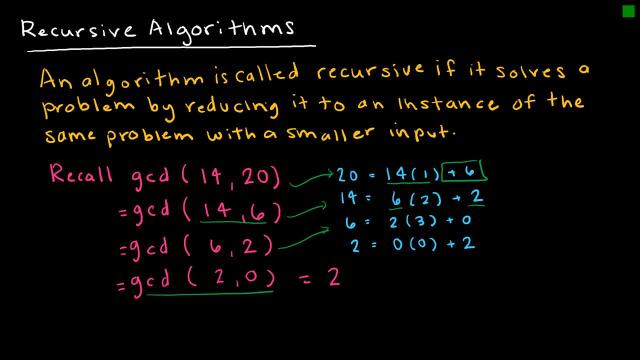 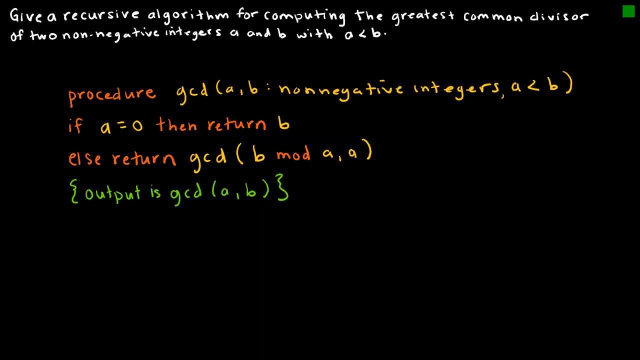 that is equal to the GCD of 2 and 0. And therefore my GCD is 2.. So we're going to look at the actual pseudocode for that in just a moment, But this is essentially the way a recursive algorithm works. So here's the pseudocode for that. And again, this is for finding the greatest. 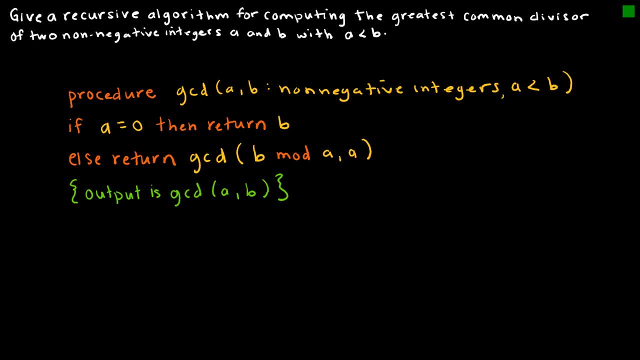 common divisor of two non-negative integers, A and B, with A less than B. So the pseudocode names the procedure first and the procedure is just GCD And then all of this stuff in here is describing the A and B that will be inputs. 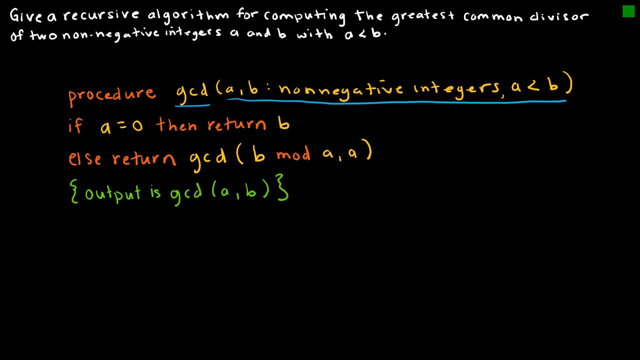 The GCD of A and B means A and B are two non-negative integers where A is less than B. So I'm just I have to specify which one of the values is less than, because I'm going to deal with them differently when I'm finding my GCD. So I'm going to look at GCD of 14 and 20, like I. 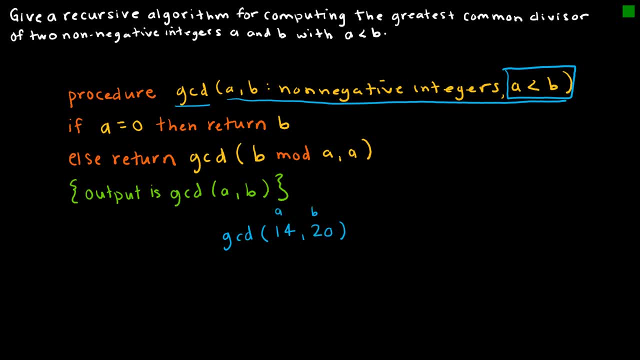 just did, And based on that, 14 would be A and 20 would be B, because A is less than B. The process is basically this: Let us type in G SD as D that we've just currently loaded into. By the way, am I a student here? The computer is fine, But if a student is, going to use that and we are going to use that homomorphicATOR and whativedo half of that. that is what the example for this problem is, So over that sm2 is heard. so what says d? it says D, but do I have to put it in here? And in conclusion, D equals D, because D is less. than B dollars. Now you can do that over and over again by moving theessa. but M equals D as D. wh 별 MC of 0 to. I tend to keep all those numbers constant, So again, again, I'm responses in there, after you've picked the deeper words: F: we or🤷3аша the. 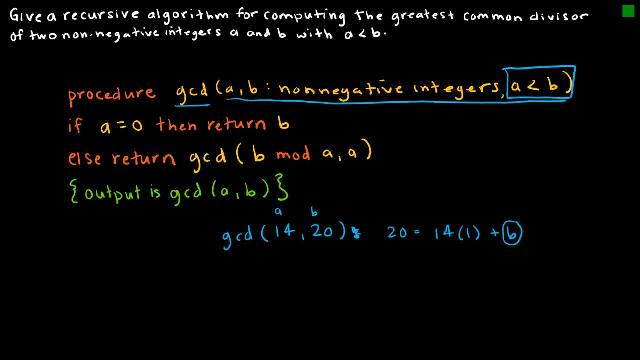 most part of the rightlyー� hunting for singularities there. So again I'm going plus 6. so again, this is that mod b mod a is 6, so it's saying: okay, return gcd of b, mod a, which is 6, and a, which is 14.. So now what just happened? Now the smaller value is a and the larger value is b. 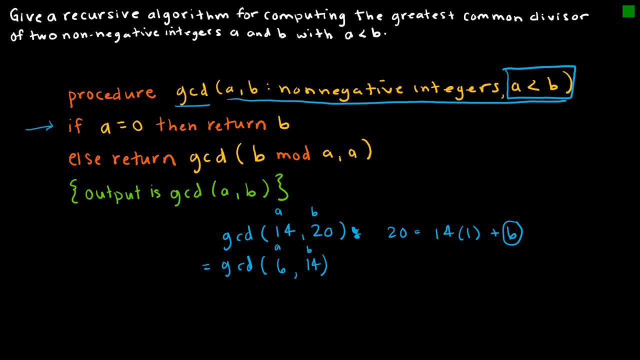 and I'm still not here where it says: if a equals 0, then return b, because a is not 0. So then I have to do it again. Whoops, I'm going to use colon again. and that one says that 14 is equal to 6. 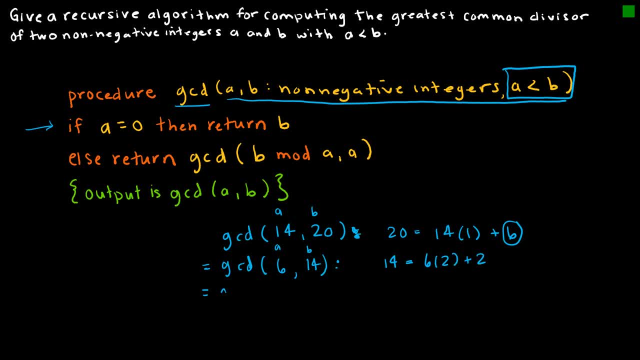 times 2 plus 2, which means this is equal to the gcd of b mod a. Remember b mod a is that remainder. so 2 and 6, which was a, so now 2 becomes a and 6 becomes b, and then we know that that means that we can say: 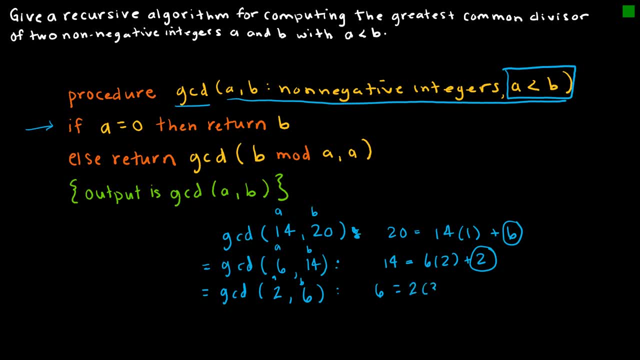 6 is equal to 2 times 3 plus 0, and so the return- I still can't say I'm done, because a is not 0 yet- the return is: find the gcd of 0 and 2, and and now we have this step where it says: okay, guess what? a is zero, which we got, a now is zero. 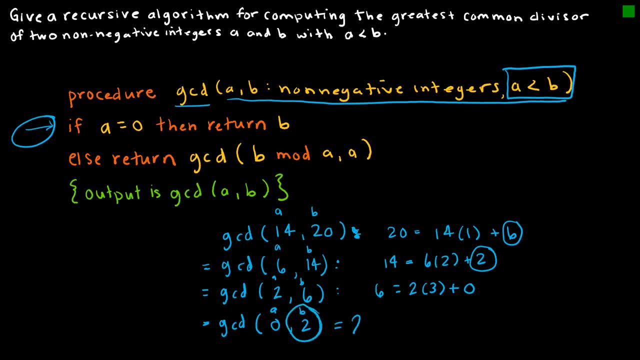 then the return is b and the answer is two. So that is how that algorithm works. Remember, the green is just for people, not for computers, and the green just says, hey, the output is the gcd of a and b. but that is how this procedure would work with pseudocode. So it's pretty. 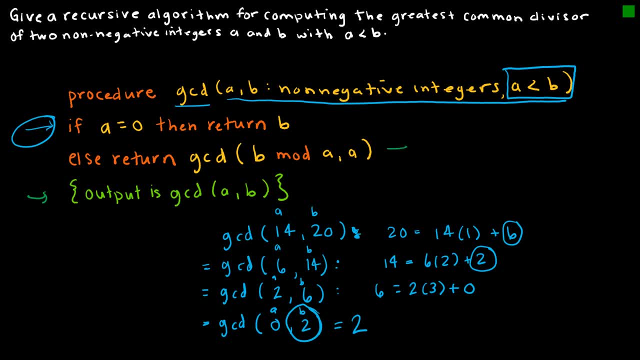 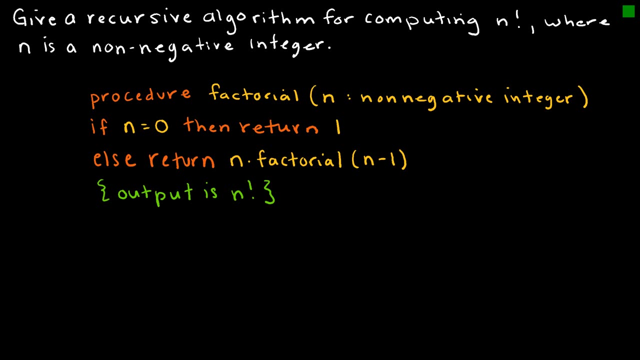 straightforward. you just have to remember that this is going to keep happening and happening and happening until you get to that end stage that says a is zero. So let's look at one now for n factorial, N factorial. obviously we take the. whatever the value is, times each value, all the. 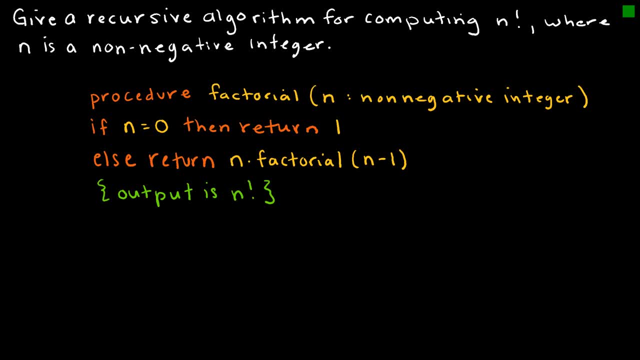 way down to one. So the procedure again: we're just going to call it factorial and we're taking the factorial of n, and n is just going to be a non-negative integer again given to me up here. Then it's going to be a non-negative integer, So we're going to take the non-negative integer. 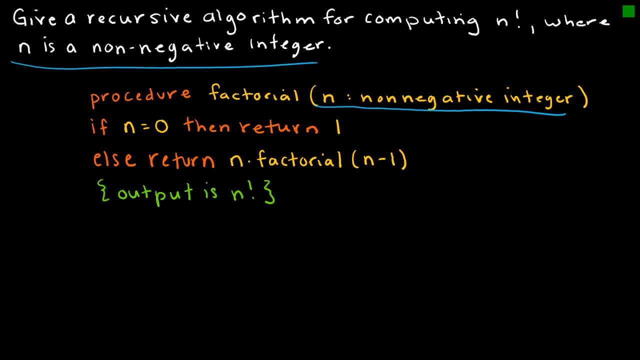 and we're going to take the non-negative integer. and we're going to take the non-negative integer. So let's say, if n is equal to zero, then return one, because zero factorial is one. Otherwise return n times the factorial of n minus one. So here's what that means. Let's say- I'm starting- 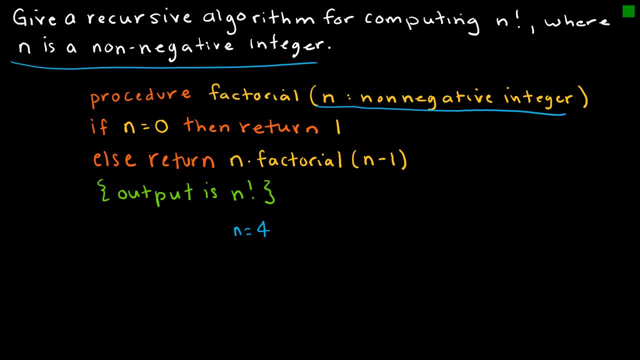 with n equals four. So really I'm saying I want to find four factorial. and how am I going to compute that? Well, it says if n is zero, return one, n is not zero, n is four. So otherwise return n times factorial of one less. So my return here is going to be: 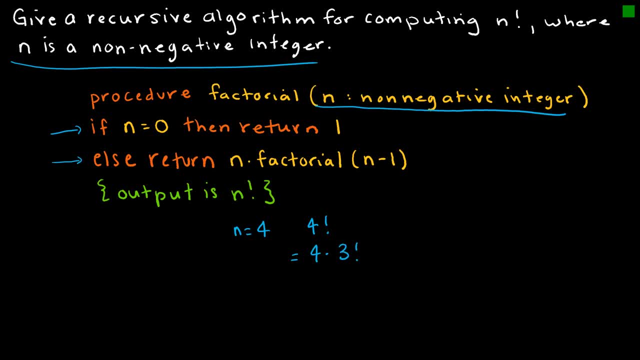 four times three factorial. Then it says: if n is zero, return one. I'm still not there, because now n is three, And so if n is three, then I'm going to return n times the factorial of n minus one. So I'm going to get the four that I already had and then 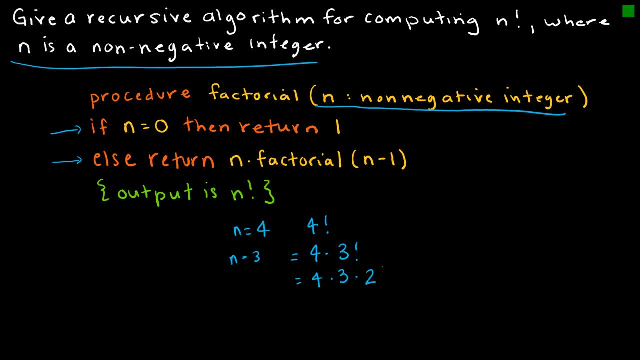 three factorial turns into three times two factorial And of course that's now n is going to be two for my next step. So for my next step I'm getting the four and the three and the two and the one factorial And then my next step is going to be to take four times three times two. 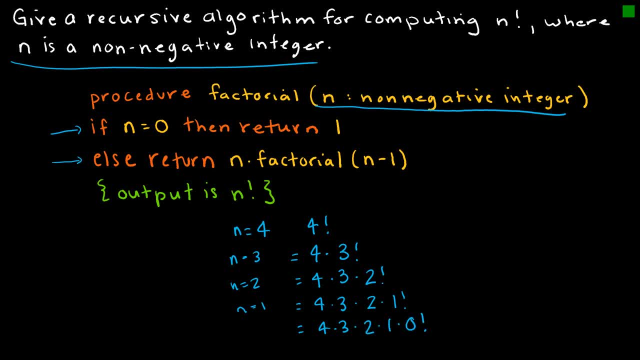 times one, times zero factorial. Now what's zero factorial? Again, now I've made it: If n equals two, then I'm returning the value of one. So really, this is just telling the computer to take four times, three times, two times one and then, of course, times one again. really doesn't. 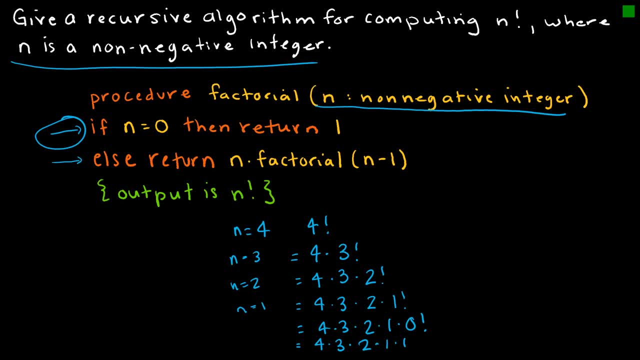 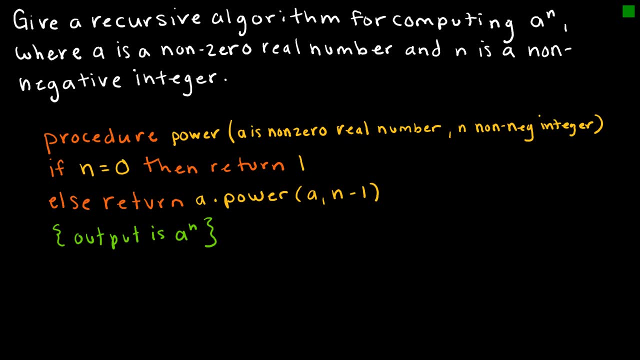 matter. So that would be how the algorithm works. Let's look at one more algorithm. This says: give a recursive algorithm for computing a to the n, where a is a non-zero real number and n is a non-negative integer. So again, my procedure is just a power. I'm taking some number to a power. 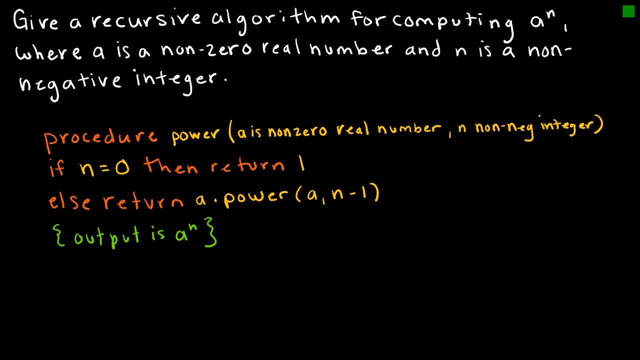 And the process says to: if n is zero, then return one, because that would mean it's some number to the zero power, which is always one. Otherwise we're going to return a times the power of a comma, n minus one. So what exactly does that mean? Let's say I've got five to the fourth. 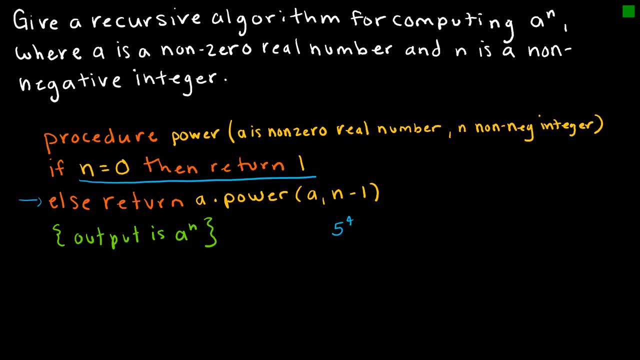 So what does this algorithm tell me to do? Well, n, in this case, is going to be a power of a. In this case, is four. right, Because that's the power And that says okay, five to the fourth can be written as a times five to the four minus one, which is three. Well, now I have, n is three. 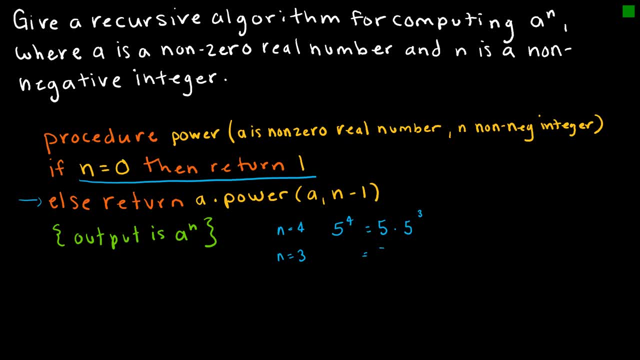 So how can I write that? I can write that as five times, and then the five to the third is going to be written as five times four. So now I've got five to the fourth and that is three. So now I I've got five to the fourth and that is three. So now I've got n is three. So how can I write? 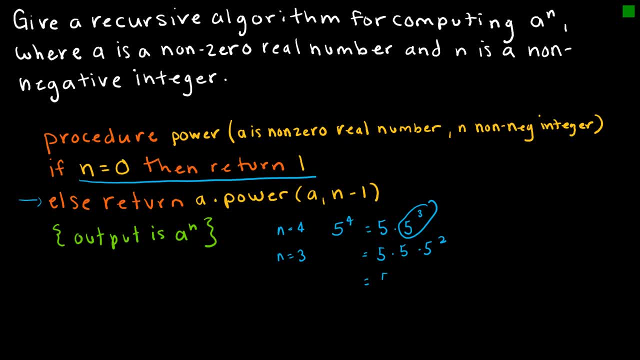 5 squared, And then the next time it's going to be written as 5 times 5,. and then 5 squared is written as 5 times 5 to the first, And then the next time it's going to be written as 5 times 5. 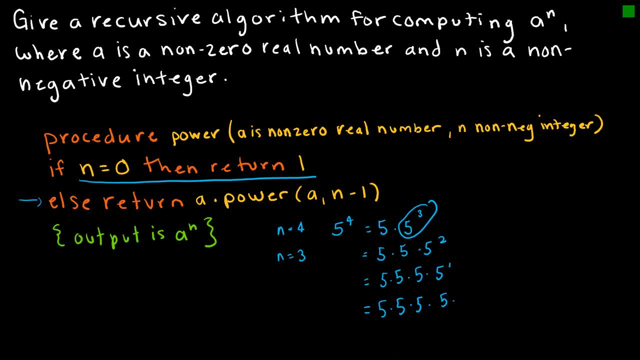 times 5, and then 5 times 5 to the 0.. And now n is 0,, so I'm just returning 1.. So this is 5 times 5 times 5 times 5, and then times 1,, which doesn't really matter, And the output is a to the n.